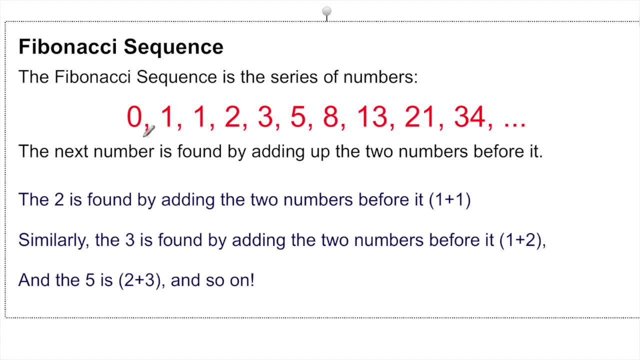 and so on and so forth. Should I go slower? 0, no, it would be an all day if I do that. Alright, so the next number. so let's take a look at the order in which these numbers are written. okay, or terms, but let's take a look. 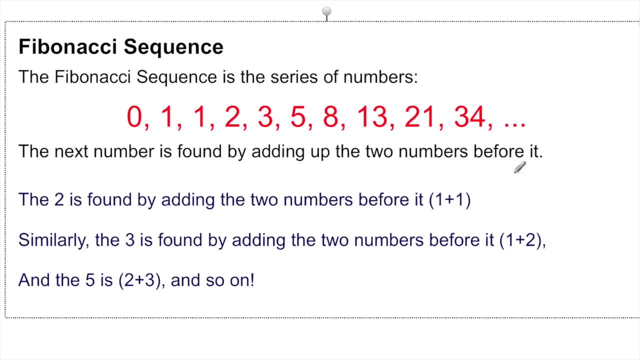 The next number is found by adding up the two numbers. So if we take number 2,, 1 plus 1 equals to 2.. Similarly- I think that's from the book, but regardless- 3 is found by adding the two numbers. 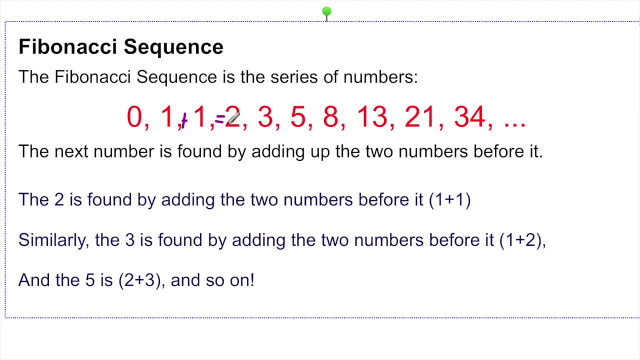 before it. So 3, 1 plus 2 equals 3, 3 plus 5 equals 8, 5 plus 8 equals 13.. Now what this is? it's basically a precursor to algebra, which we're going to be doing. 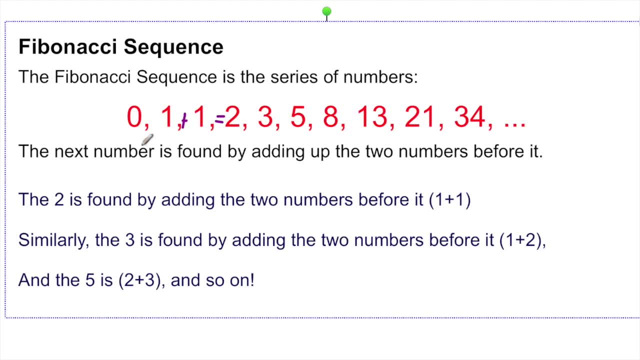 over the next couple of weeks. Okay, but you just have to understand this and, again, I will go forward and give examples of this in class and we will review it, so don't worry about it Now, this is a rule and we will be using this rule before. hey, check that out. 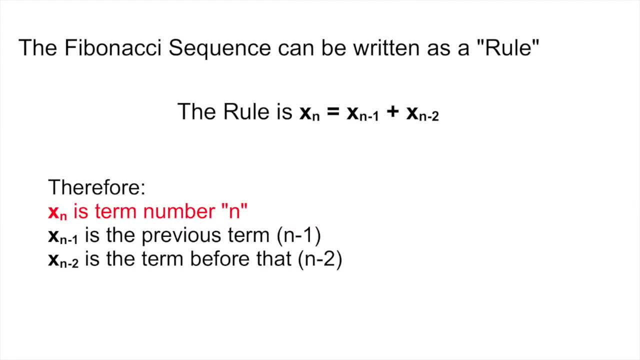 Anyway, we will be using this rule just to understand this. okay. We don't really like I've never used a rule before with this, but it's just interesting to have Write it down. okay, because we will be using something like this later on in a few lessons. 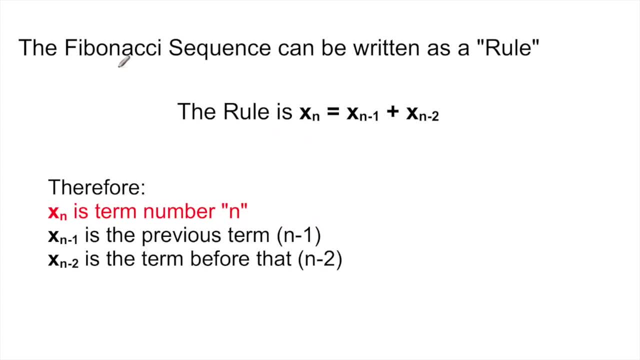 Okay, So now next week, look out for something like this. Okay, so the Fibonacci sequence can be written as a rule: okay, X, n, number there's, your variable equals. so you, basically, your third number will equal to the first number plus the second number. 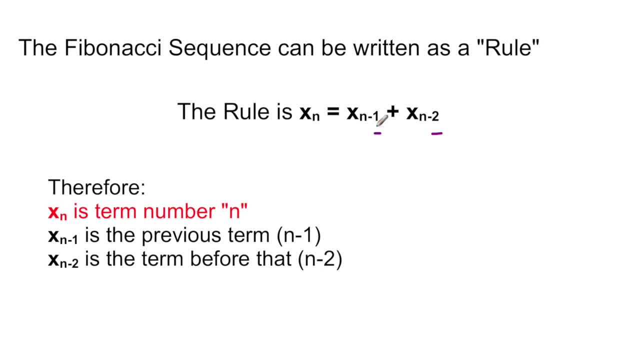 See that. First number. second number: alright, Minus. now the reason minus is because of the previous term. okay, So the previous term plus the previous term before that. That's where you get the two from. So the previous term plus the previous term before that. 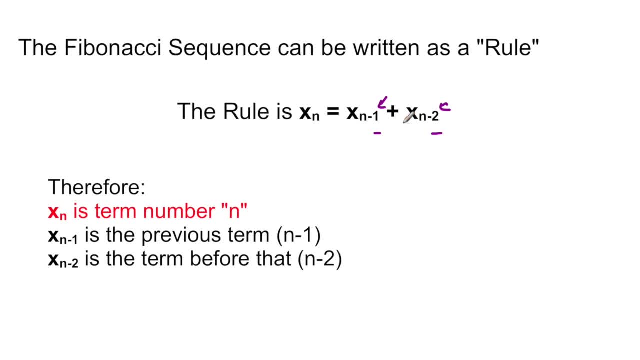 Don't worry about this, This is really complex. Just write it down, Just have it, Just know it, Just see it, Look at it. Write it down, okay, I don't expect you to know this, but just interesting to have. okay, just so you can.